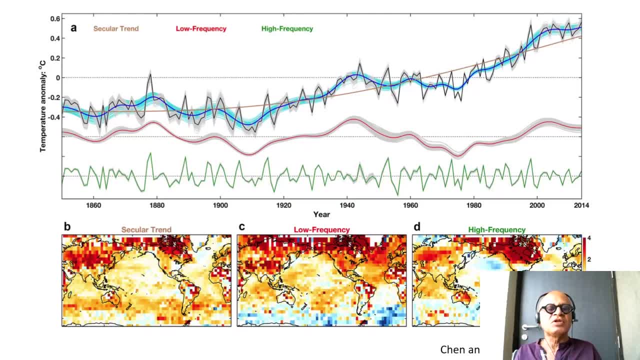 patterns. that's not easy to do. we will see a little bit more about that later, so I took the figures from elsewhere and not from the book chapter, but the message is the same. what you do is use things like statistical tools of spectral analysis, empirical orthogonal functions. 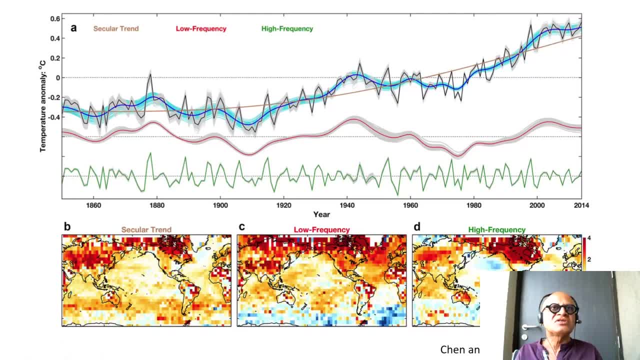 multi-channel singular spectrum analysis and so on, to extract the various patterns. so if you have a time series of sea surface temperatures or surface temperatures going from, let's say, 1850 to here, 2014, it has grid distribution, spatial distribution, latitude, longitude latitude and time distribution. these statistical tools will let you extract the 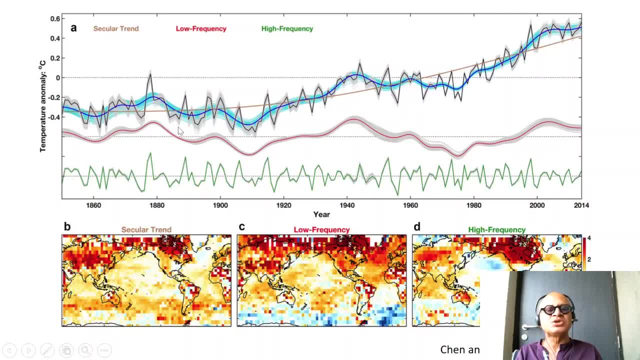 low frequency variability here. so that shows you the trend or the decade-to-decade variability. but again the question is how the decade-to-decade variability is going to affect the global warming. so for those of you who are familiar with the global warming strategy, it tracks the, the. 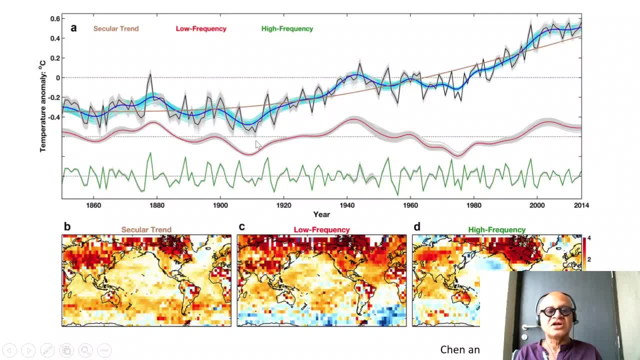 global warming pattern from 10 years to decade, or from 10 years up to 5th decade. the variable was modified by greenhouse gases and global warming and it extracts this low frequency variability which has no trend in it. so, in terms of temperature anomaly, you can see that this 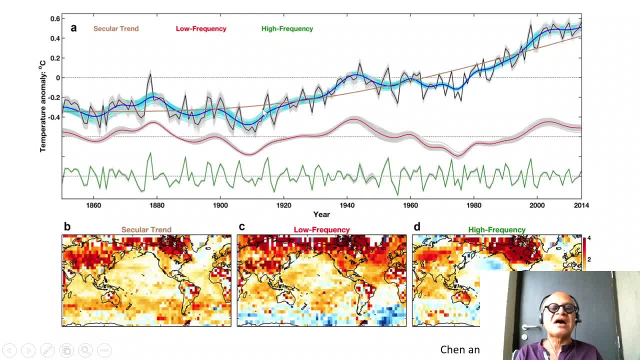 pattern is corresponding to this particular time series. so if you multiply this time series to this, you will get the value for that particular year. for example- and this is the low frequency variable- in a much more than one year, you can follow my example of the value of the time as a. 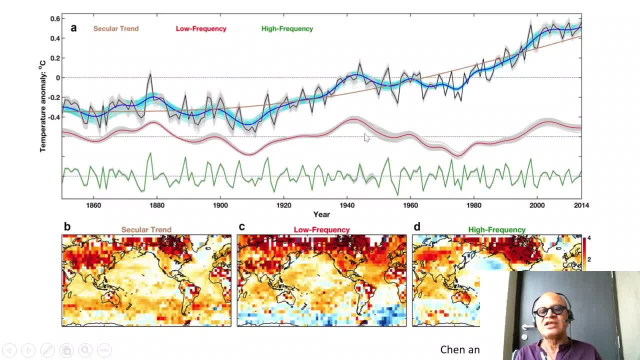 variability, which is a time scale of decade or two, depends. so from the data you can extract these time scales and then you want to look for processes or modes of variability or mechanisms which generate these low frequencies, always keeping in mind that atmosphere has no memory, so it cannot produce low. 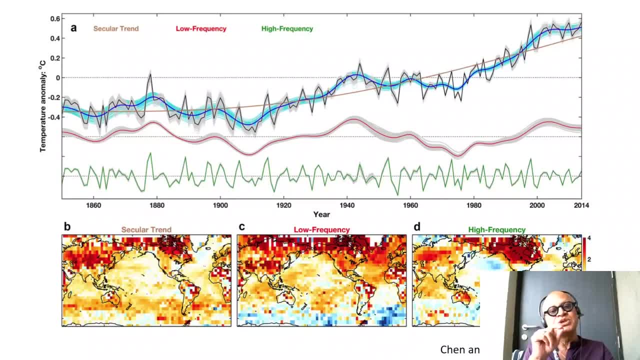 frequencies. so it has to come from glacier melt, vegetation changes or ocean changes, so ocean can control coupled variabilities at low frequencies. and then this pattern here is showing this high year-to-year variability, the high frequency and, for those who know what this is, this kind of warming or cooling. 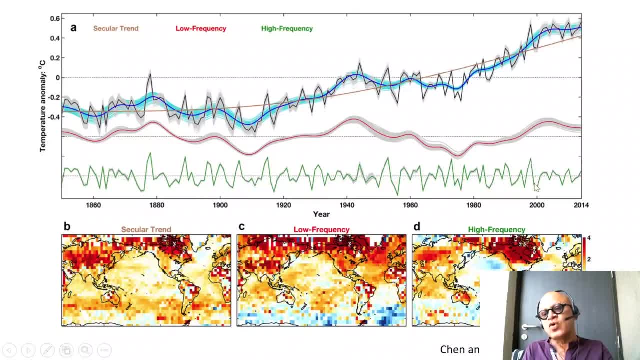 so remember that this time series is positive or negative. so remember that this time series is positive or negative. so remember that this time series is positive or negative. so when you multiply, you will get either positive anomaly or negative anomaly. it's the same for all of them. okay so, and there is statistical significance. 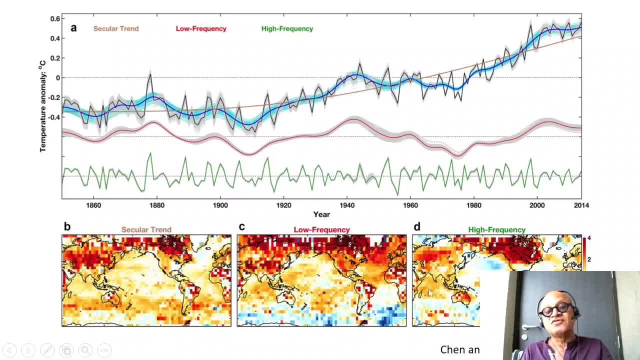 issues in the regions where there is no color. okay, you have to be careful that there is often not enough data to say confidently that there is a change there. okay, so this pattern here corresponds to what we call the El Nino, or La Nina or El Nino Southern. 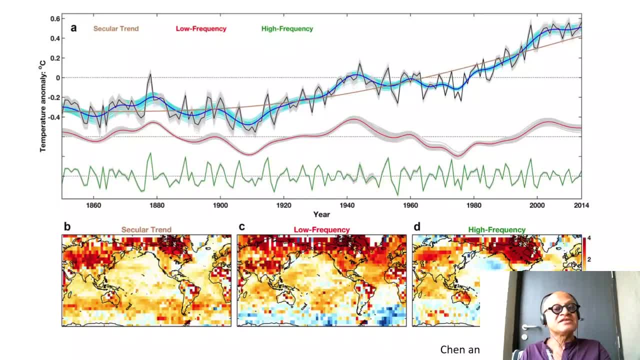 Oscillation. I have detailed podcasts on El Nino and La Nina and so on that you can look up, but this is the year to year variability. so El Nino happens here in the Pacific, sometimes warming or cooling around, warming around the dateline, sometimes warming, extending all the way to the coast of North and South America. 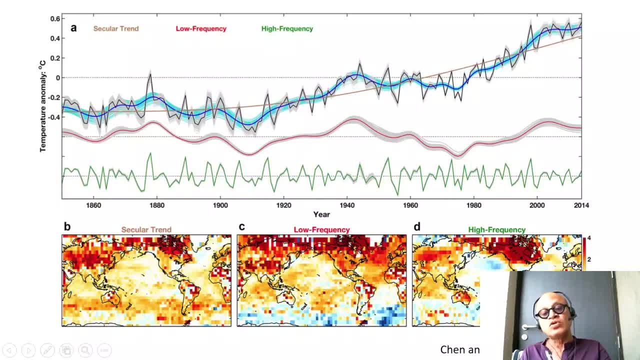 climatologically, if you remember, the temperatures are cold here, Galapagos is cold and cold. is that the Pacific is really warm and cold and cold? you know, upwelling primary production or photosynthesis, rich biodiversity, whereas here you have warm waters, warm pool moving with the sun, coral reefs, great barrier reef and so on and so forth. 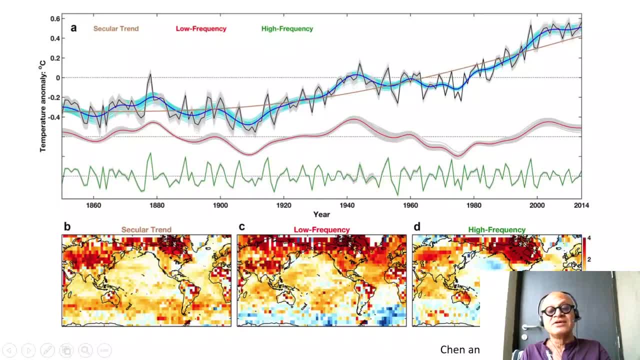 lot of rain, there's no rain here, and so on. right, So these are the predominant modes or patterns of variability. There are other variabilities, obviously in the Atlantic, at the high latitudes, in the Indian Ocean, and so on, and you also see that the so-called secular 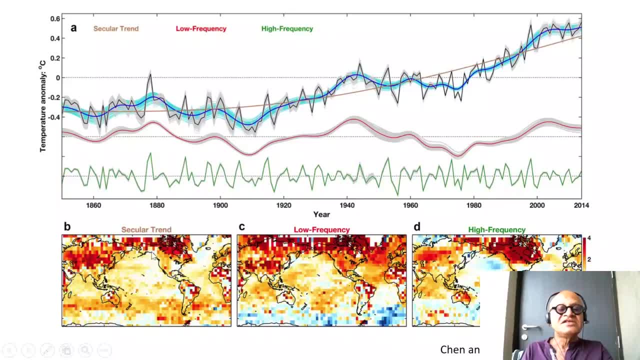 trend, which means it's over a certain period, is higher at high latitudes here in the Arctic than in the tropics, for multiple reasons because there is ice albedo feedback happening here right. If you warm a little, you melt ice and snow and you reduce the albedo, absorb more energy. 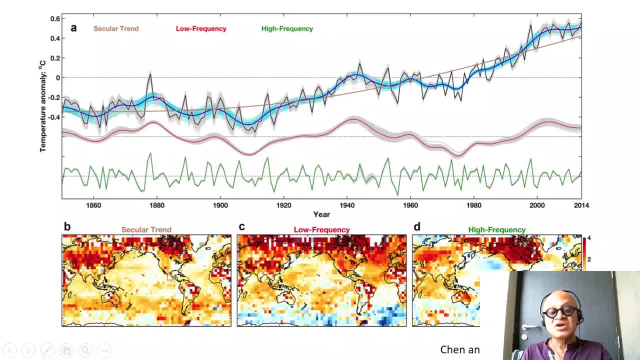 so you get more warming. In the tropics temperatures are warmer, so warming- little warming- can produce atmospheric convection which tends to take away the energy, and so on and so forth. So the consequences of warming will also be different. So when we talk about global warming, 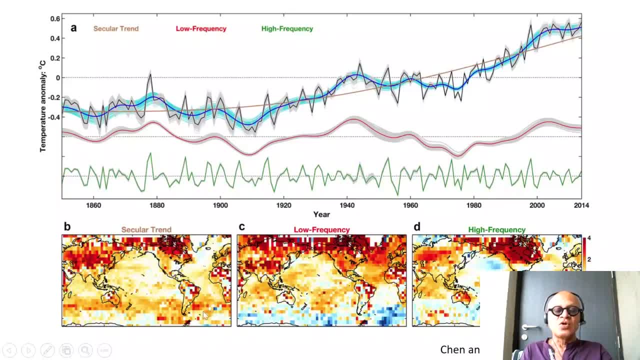 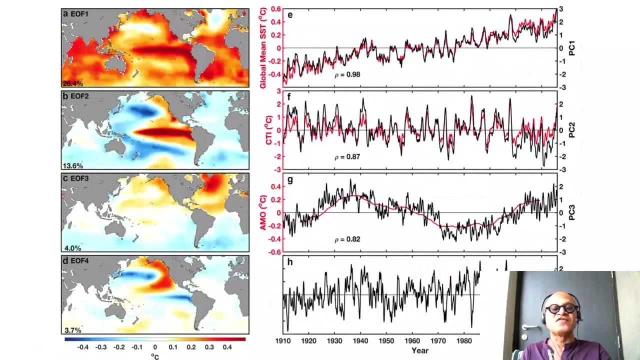 we should always remember that we are averaging over these cooling here, cooling or no warming here, more warming here, less warming here, and so on. So the question is: how are these natural modes being modified by these additional warmings happening because of human activities? 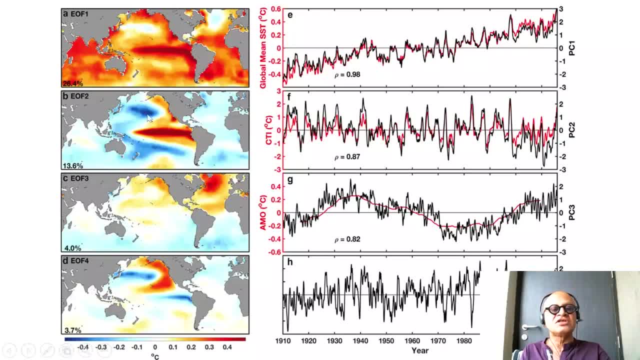 So this is another way to look at it. This is looking at sea surface temperatures, now no land temperatures. Global mean sea surface temperature shows a warming trend, so it's showing the data itself and the time series, or the principal component of the empirical orthogonal. 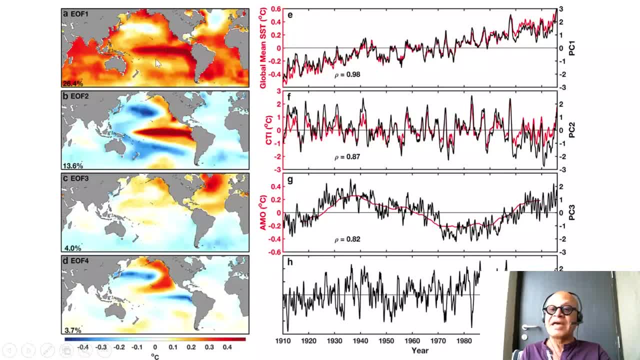 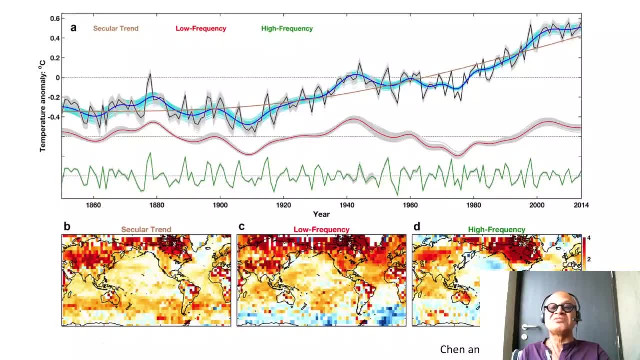 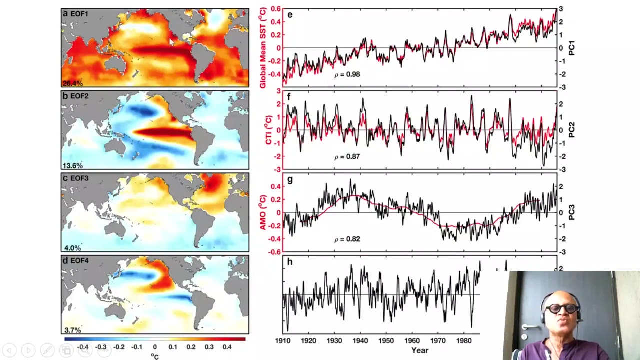 function used to extract the dominant pattern. The same thing here. These are the time series or the principal components, or the canonical modes, canonical correlations, CCAs, and these are the spatial loading or the spatial pattern. So you have to multiply this to this to get the answer. So there is a whole debate about 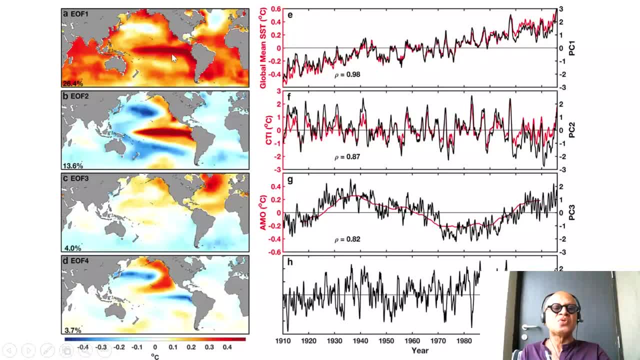 whether global warming pattern should look like El Nino or not and so on, which we won't get into. But the second EOF captures the interannual variability, or the El Niños and the La Niñas. So El Niño is when it's warm here and La Niña is when it's cold here. 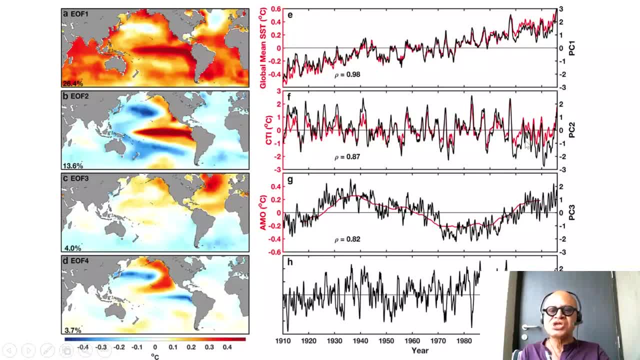 And you can see that there are apparent changes in the frequency, duration, amplitude and so on. But it's not clearly known whether that's natural variability or modulation by the global warming- Complicated things. So this shows another pattern called the Pacific Decadal Oscillation, which you can see has some similarity to the El Niño pattern. 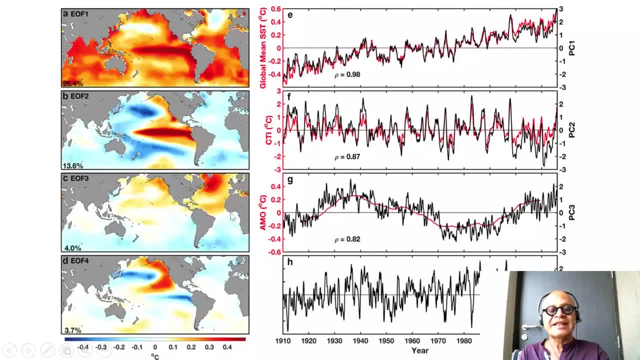 So there is this AMO pattern- Atlantic Multidecadal Variability- which has a huge spatial loading here With a different timescale than the Pacific Decadal Oscillation. So unless we know the processes that select these timescales, it is hard to know if they are oscillations or they are episodic events. 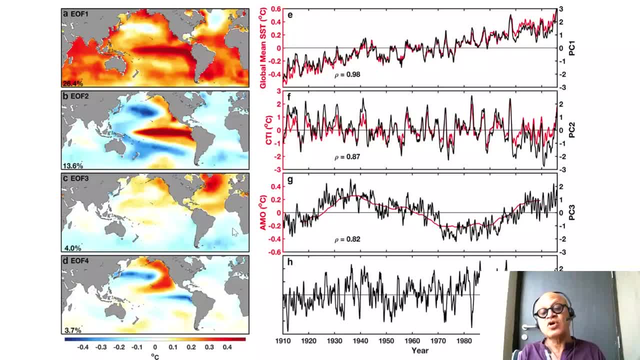 Because the data is not long enough. If you want to call this an oscillation, then you need at least two cycles to be extracted from the data, And you can see that we barely have one cycle here. PDO offers multidecadal. 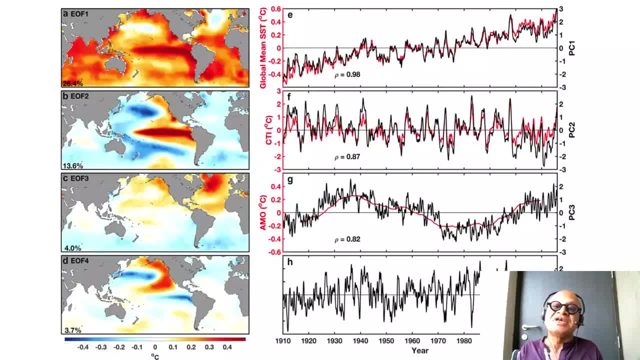 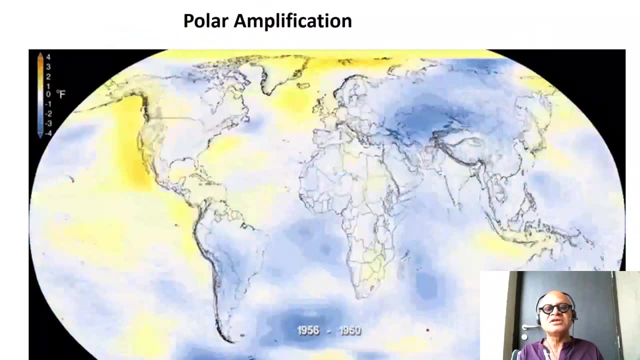 But we still don't know what the mechanism is which would produce this timescale and this pattern. Some people argue that it is related to the El Niño and La Niña itself. So complications, but we know a lot And this shows a good way to look at polar amplification. 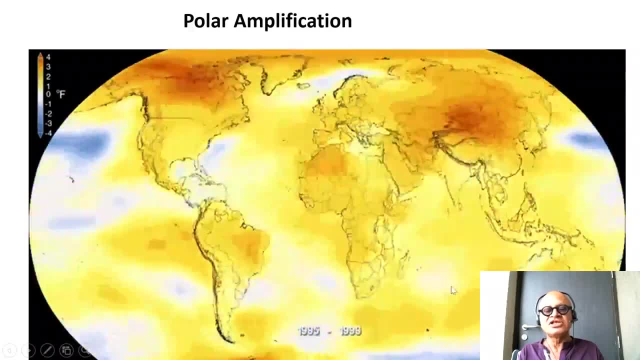 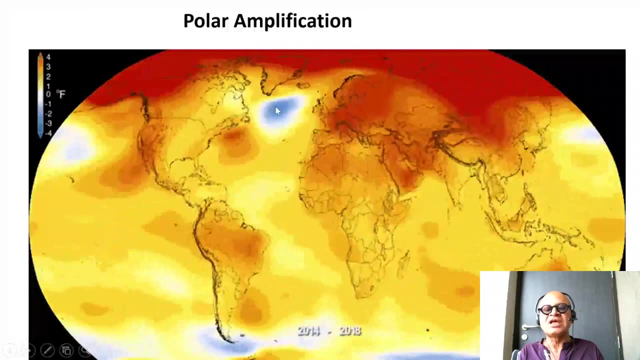 So it starts in the 1880s, I think, And you can see that lots of negative blue colors in the beginning end up becoming oligocyanins, Almost all red, with some exception here, And the polar amplification is very clearly seen. 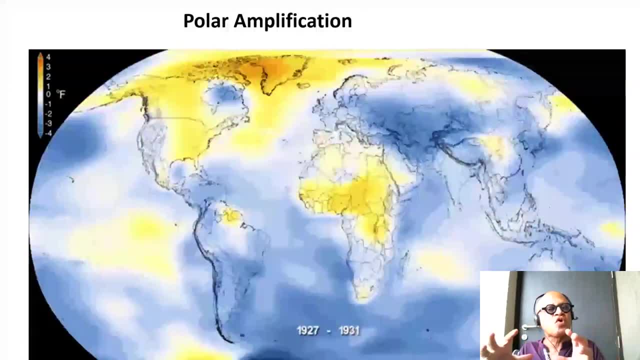 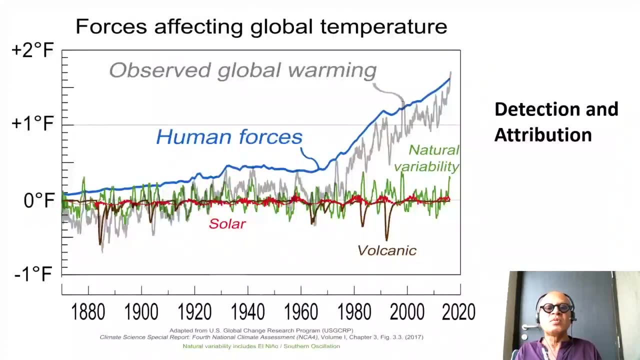 So natural variability is now happening in a warmer and warmer climate. So the question again, to repeat myself, is: how is global warming affecting natural modes of variability? How can we say for sure that global warming is happening? That's what gets us into detection and attribution. 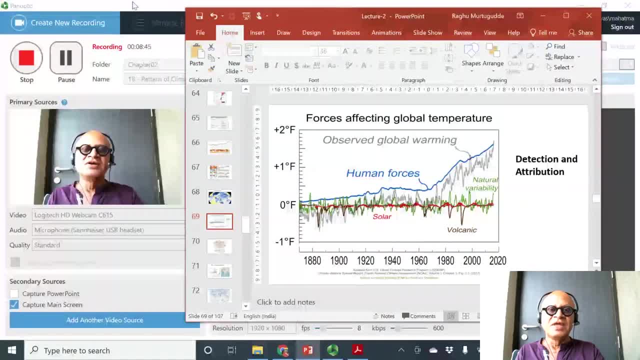 Which I will do In the next podcast. okay, So we have very good theories for things like El Niño and Monsoon, even though they are not complete. We can explain a lot of things about them, But lower frequencies like PDOs, AMOs, have some work left to do. 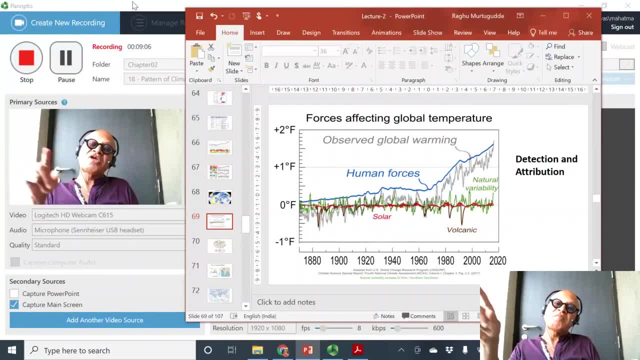 And then the question is: if there is a warming on top, how can we be sure that it is in fact related to human activities, human behavior, human behavior, How can humans deal with the warming and human emission of greenhouse gases and so on?